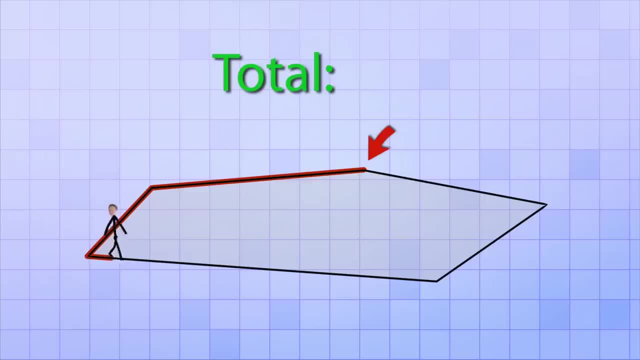 Imagine starting at one of the polygon's vertices and then walking along each side until you got all the way back to the point that you started from. The total distance you traveled would be the perimeter of that shape In this case, if the length of each side of the polygon was 10 meters. 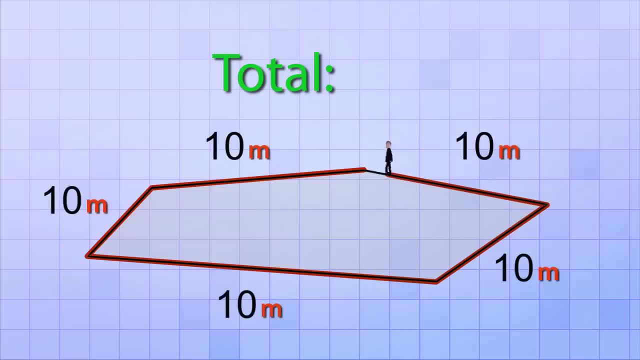 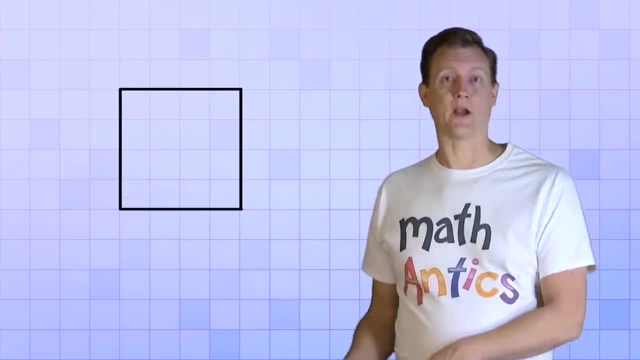 the total length you would travel along all five sides would add up to 50 meters. Another good way to see what perimeter is is to imagine that you could take a shape like this square and break it at one of its corners. Then you could unfold the shape until it formed a straight line. 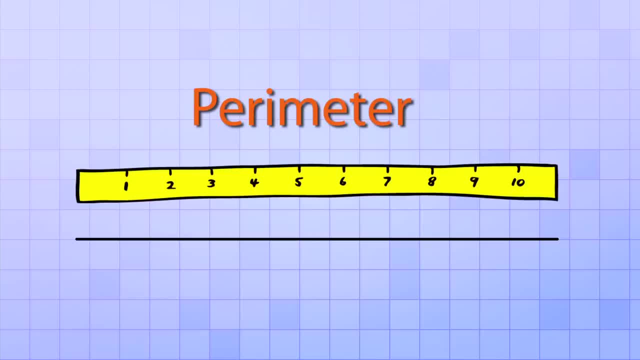 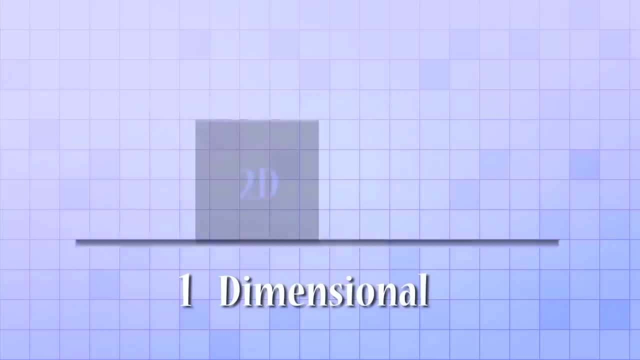 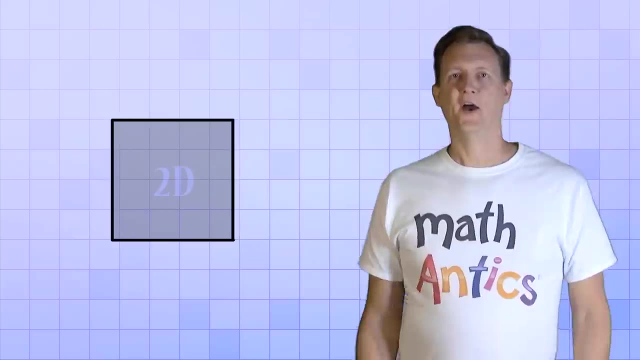 The length of that line is the perimeter of that shape. The length of that line is the perimeter of that shape. Doing this helps you understand why perimeter is a one-dimensional quantity, even though it applies to two-dimensional shapes like this square. It's one-dimensional because it's the distance of the lines that go around the two-dimensional shape. 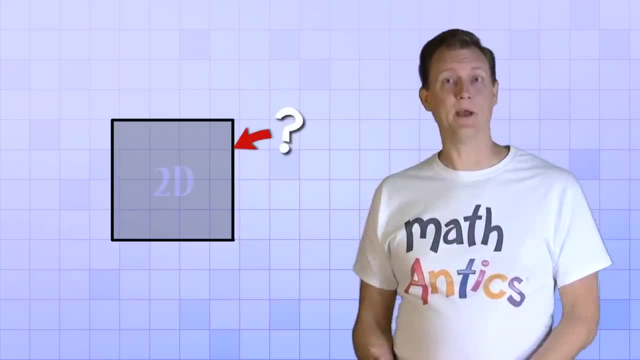 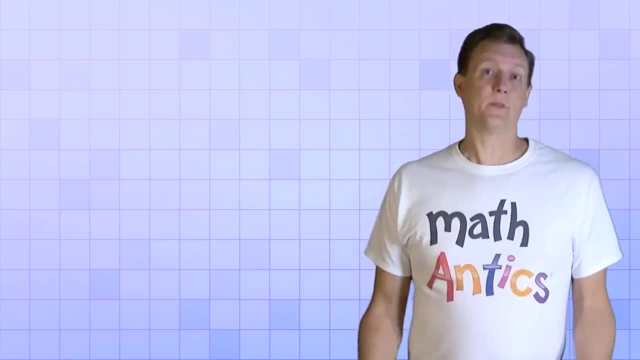 Okay, so now that you know what perimeter is, how do we measure or calculate it for different geometric shapes? Well, that depends on the shapes. Finding the perimeter of shapes that have curves, like circles or hearts or things like that, can be tricky. 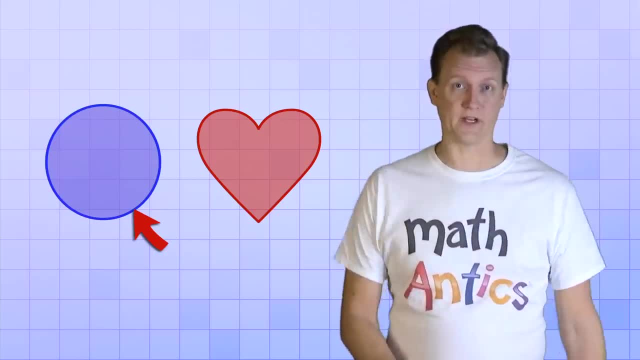 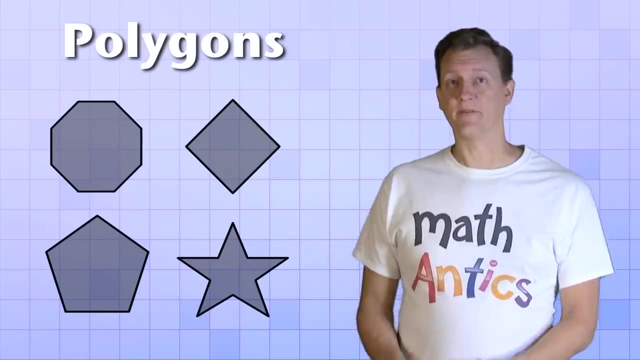 In fact, we'll wait and talk about the perimeter of a circle in another video. In this video, we're just going to focus on how to find the perimeter of polygons. Since polygons are made from only straight sides, it's easy to find their perimeter. 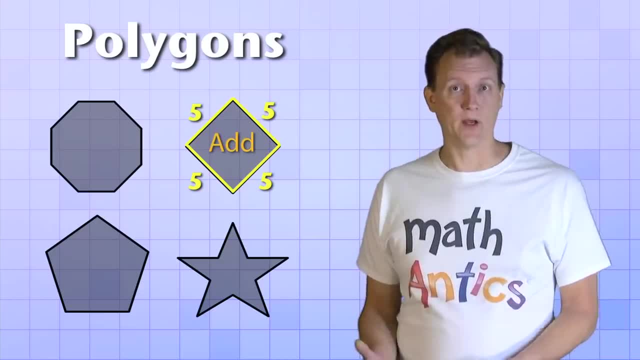 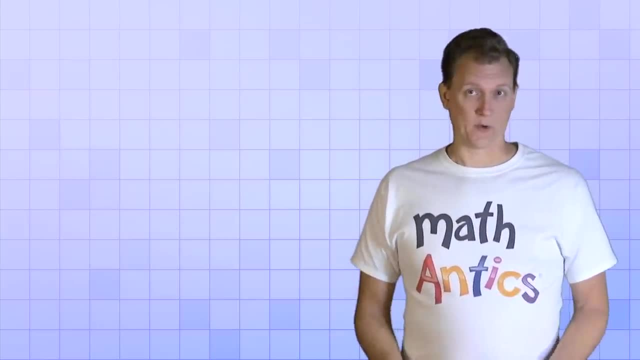 If you know the length of each side, all you have to do is add them up and the total length you end up with is the perimeter of the polygon. Let's try doing that with a few examples so you see how it works. The first polygon we'll try is a triangle. 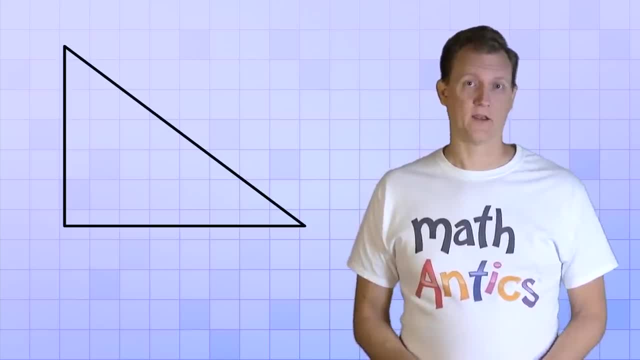 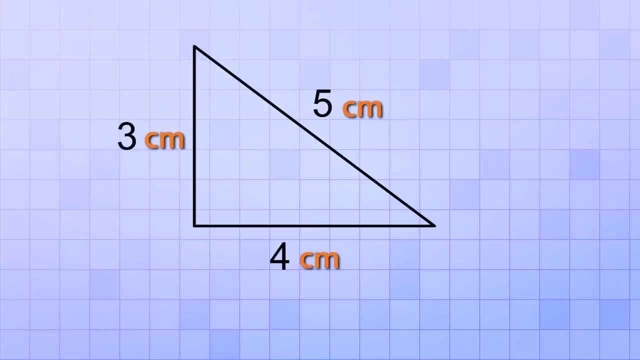 This triangle has three sides that are each a different length: 3 centimeters, 4 centimeters and 5 centimeters. Now, to find the perimeter of the triangle, all we have to do is add up the lengths of those three sides. 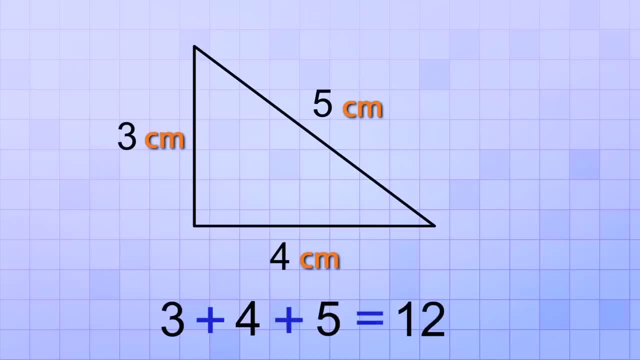 3 plus 4 plus 5 equals 12.. But don't forget, it's not just 12, it's 12 centimeters. Always remember to also put down the units of the perimeter. Okay, that was easy, Let's try another one. 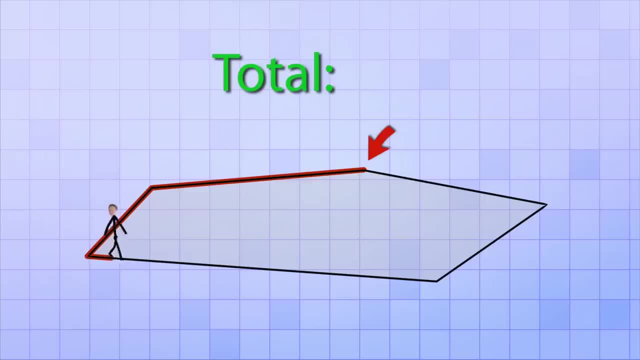 Imagine starting at one of the polygon's vertices and then walking along each side until you got all the way back to the point that you started from. The total distance you traveled would be the perimeter of that shape In this case, if the length of each side of the polygon was 10 meters. 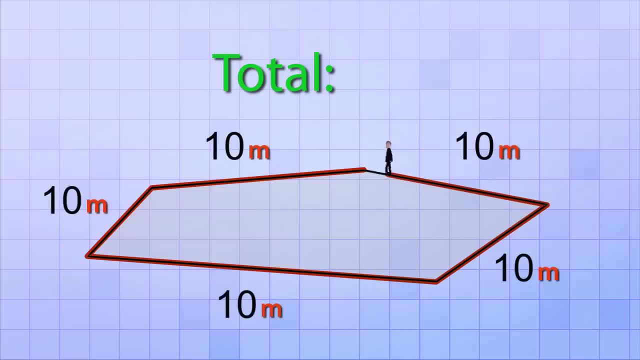 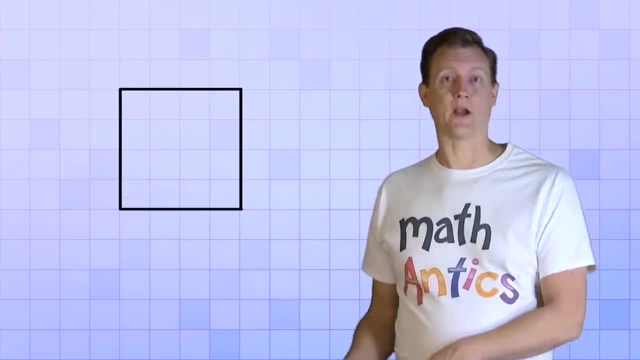 the total length you would travel along all five sides would add up to 50 meters. Another good way to see what perimeter is is to imagine that you could take a shape like this square and break it at one of its corners. Then you could unfold the shape until it formed a straight line. 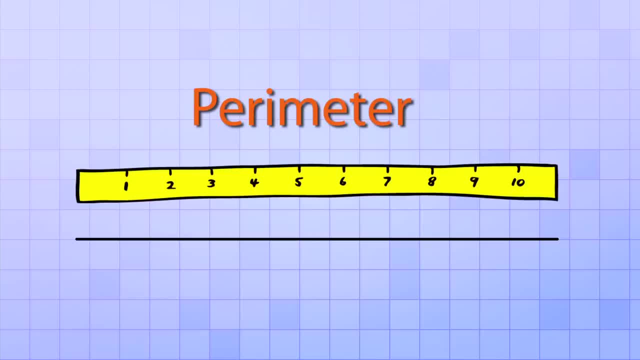 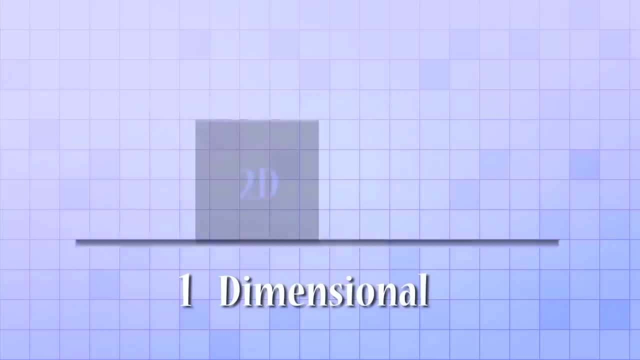 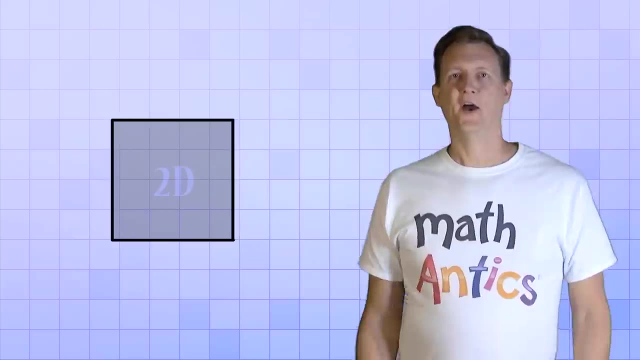 The length of that line is the perimeter of that shape. The length of that line is the perimeter of that shape. Doing this helps you understand why perimeter is a one-dimensional quantity, even though it applies to two-dimensional shapes like this square. It's one-dimensional because it's the distance of the lines that go around the two-dimensional shape. 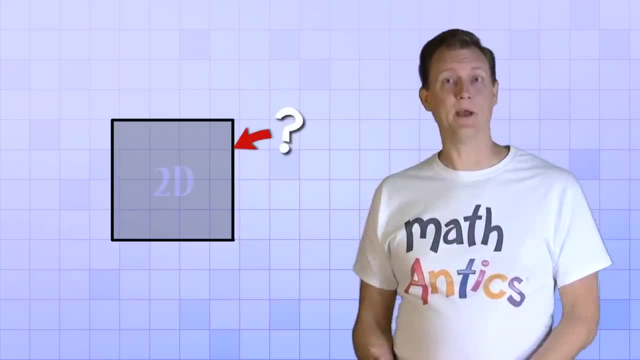 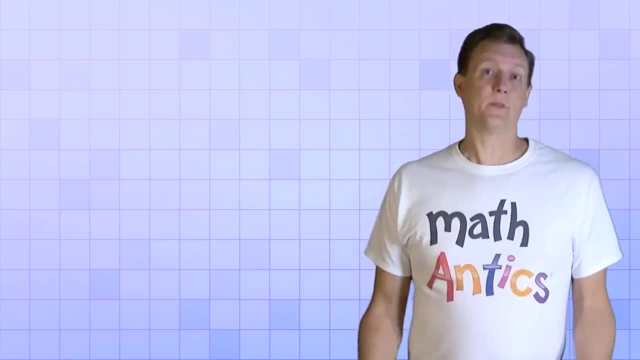 Okay, so now that you know what perimeter is, how do we measure or calculate it for different geometric shapes? Well, that depends on the shapes. Finding the perimeter of shapes that have curves, like circles or hearts or things like that, can be tricky. 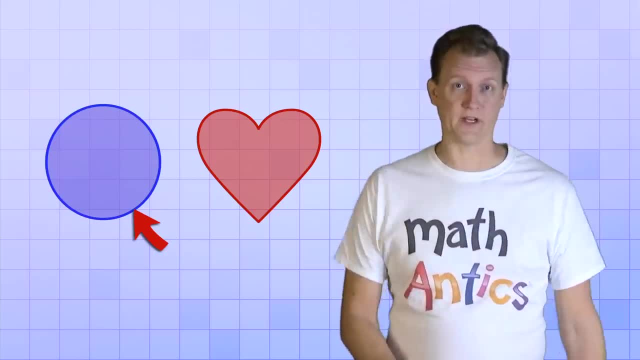 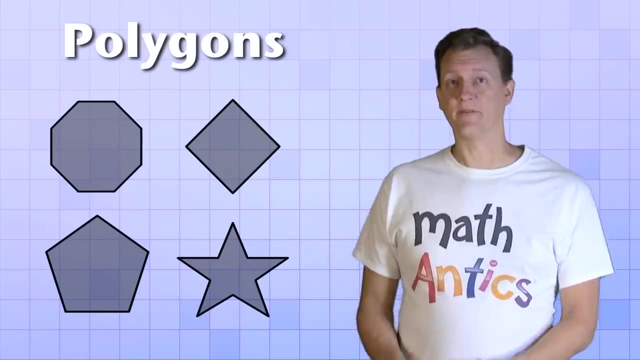 In fact, we'll wait and talk about the perimeter of a circle in another video. In this video, we're just going to focus on how to find the perimeter of polygons. Since polygons are made from only straight sides, it's easy to find their perimeter. 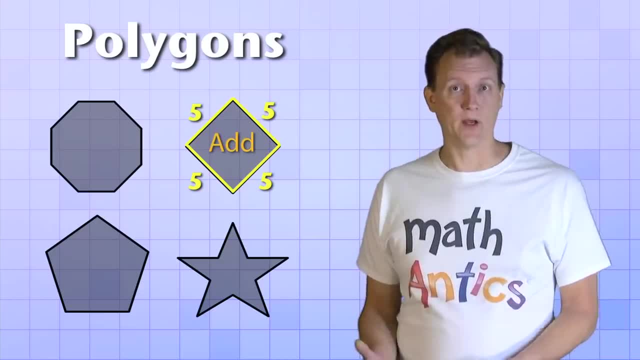 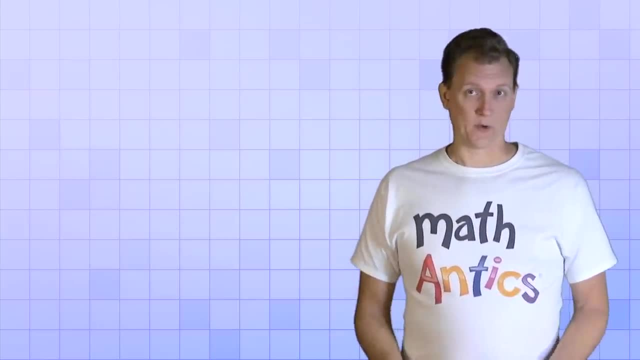 If you know the length of each side, all you have to do is add them up and the total length you end up with is the perimeter of the polygon. Let's try doing that with a few examples so you see how it works. The first polygon we'll try is a triangle. 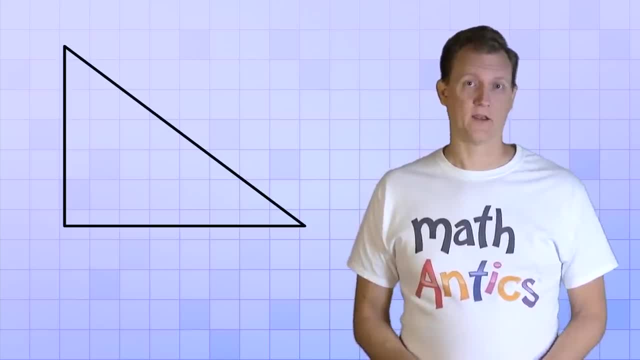 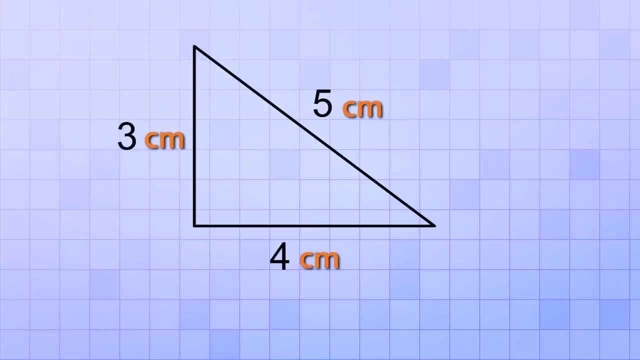 This triangle has three sides that are each a different length: 3 centimeters, 4 centimeters and 5 centimeters. Now, to find the perimeter of the triangle, all we have to do is add up the lengths of those three sides. 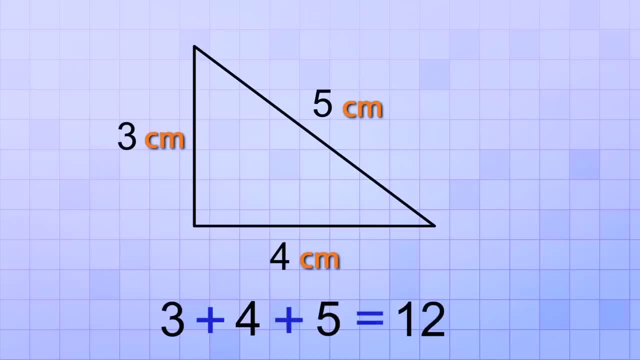 3 plus 4 plus 5 equals 12.. But don't forget, it's not just 12, it's 12 centimeters. Always remember to also put down the units of the perimeter. Okay, that was easy, Let's try another one. 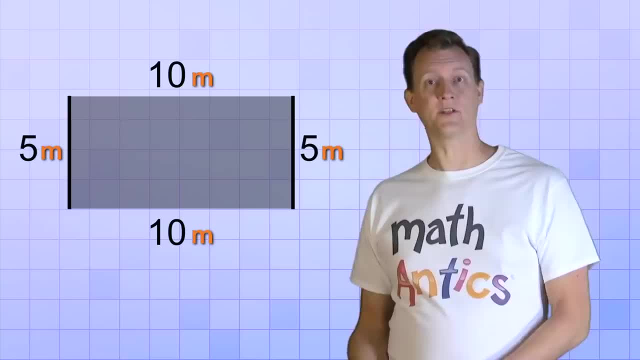 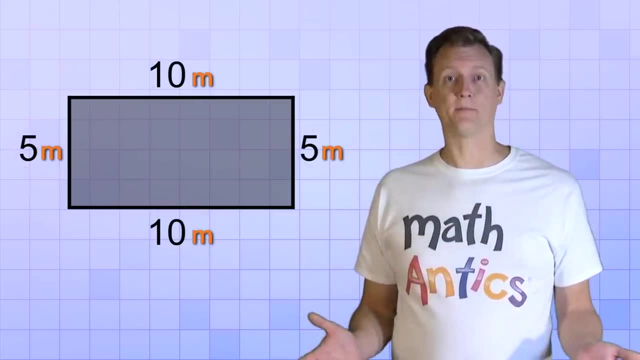 This time our polygon is a rectangle and you can see that the shorter sides are each 5 meters long and the longer sides are each 10 meters long, So let's add them all up. We can add up the sides in any order we want to. 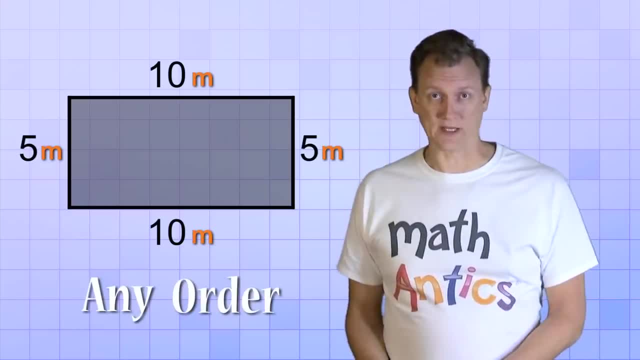 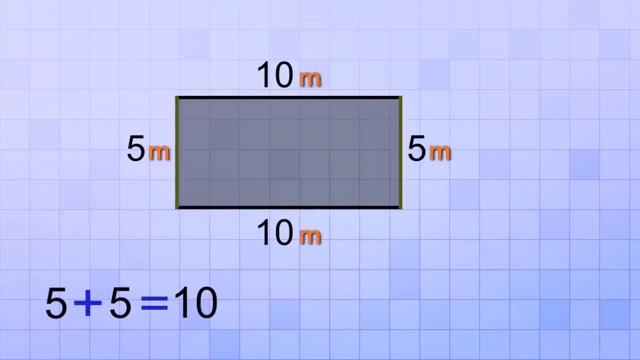 as long as we don't forget any sides or accidentally count any of them twice, And I think I'll add up the two short sides first: 5 plus 5 equals 10.. Next I'll add up the two longer sides: 10 plus 10 equals 20.. 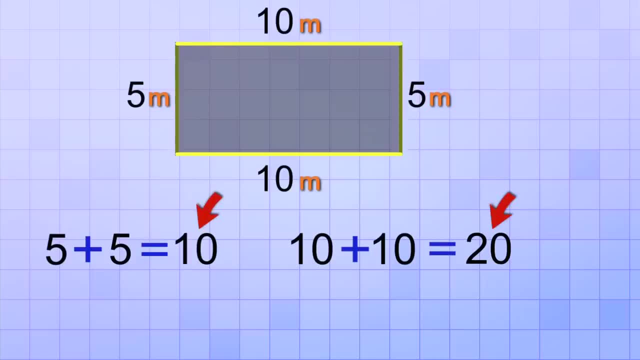 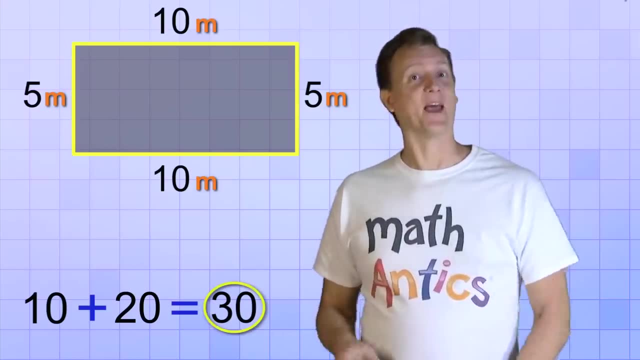 And now, if I add up those two answers, I'll get the total for all four sides. 10 plus 20 equals 30. So the perimeter of this rectangle is 30. Meters- Ha, You thought I was going to forget my units, didn't you? 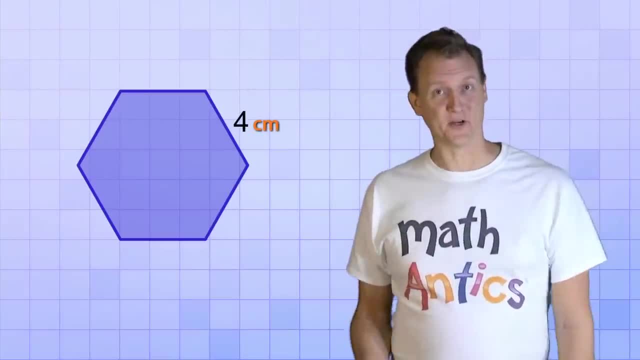 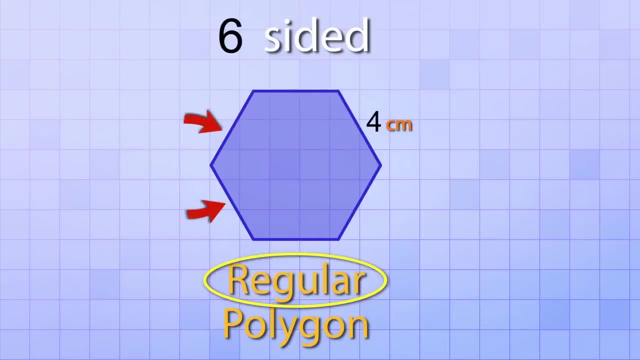 Not this time. Ah, here's another good example. This is a six-sided regular polygon. A regular polygon means that all its sides are exactly the same length, And that's good, because this diagram only shows the length of one side: 4 centimeters. 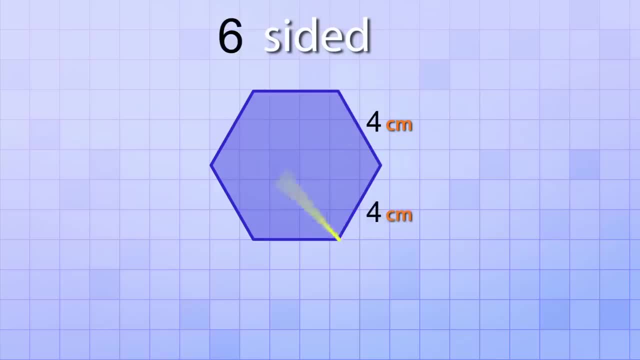 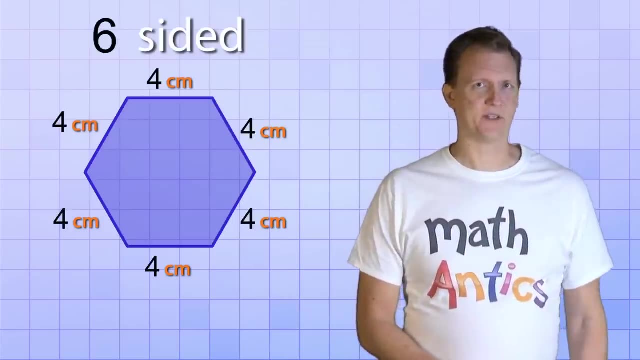 But since the polygon is regular, we know that all the other sides are also 4 centimeters long. Now we could just add up all the sides, like we did before, but since they're all the same, we can use multiplication as a shortcut. 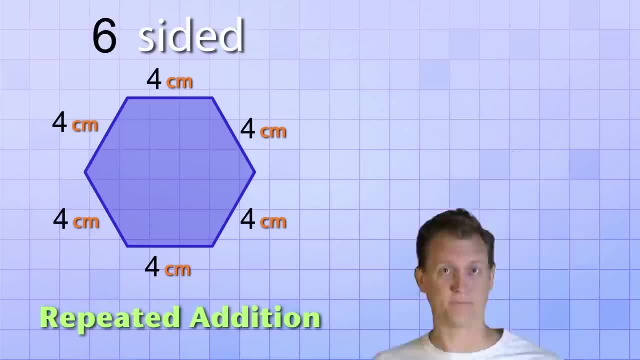 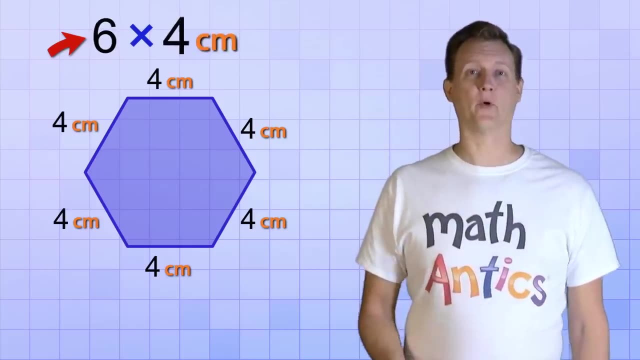 That's because multiplication is really just repeated addition. All we have to do is multiply the number of sides- 6, by the length of the sides- 4 centimeters. 6 times 4 equals 24.. So that means the total perimeter of the polygon is 4 centimeters. 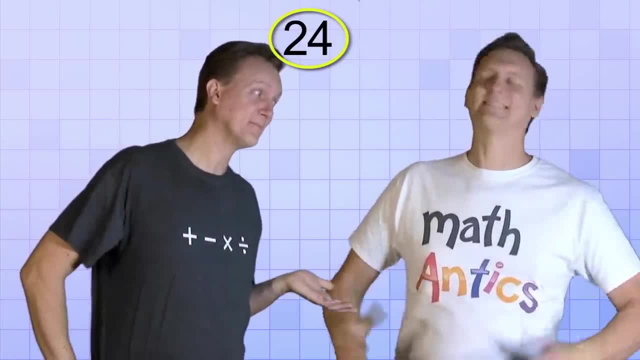 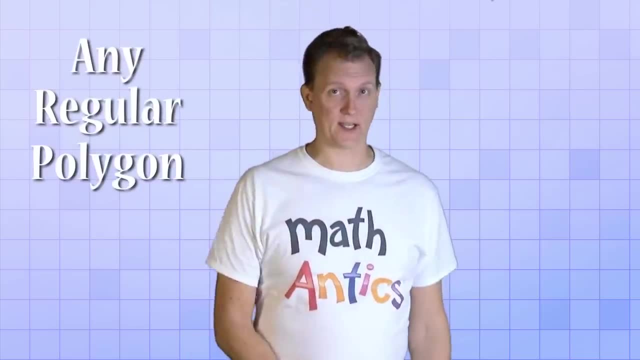 So the total perimeter must be 24.. 24, what Centimeters? That's better, Oops. And this formula works for any regular polygon, no matter how many sides there are. If the sides are all the same length, you can just multiply the number of sides by the side length. 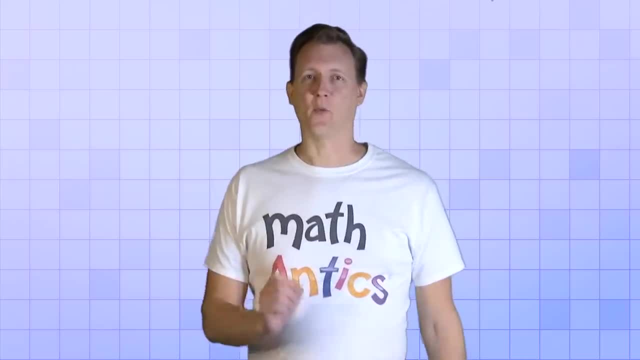 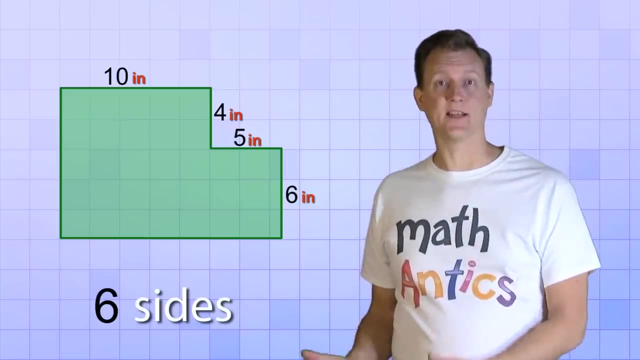 and you have the perimeter. Okay, let's try one more example. This polygon also has 6 sides, but it's not a regular polygon. The sides are different lengths, and this one's really tricky because they only show us the length of 4 of the sides. 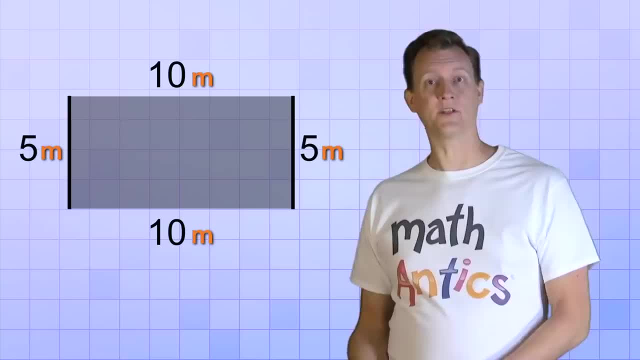 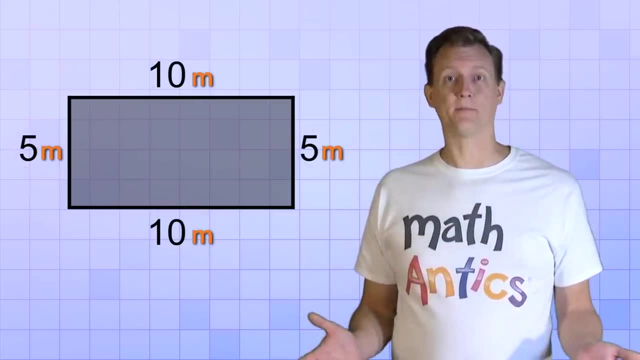 This time our polygon is a rectangle and you can see that the shorter sides are each 5 meters long and the longer sides are each 10 meters long, So let's add them all up. We can add up the sides in any order we want to. 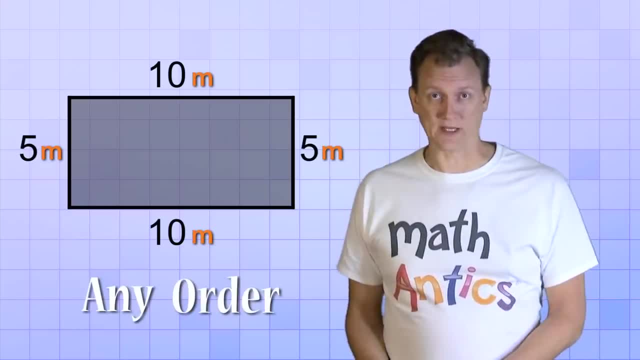 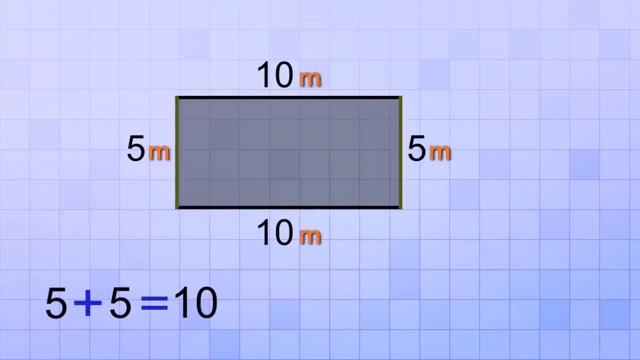 as long as we don't forget any sides or accidentally count any of them twice, And I think I'll add up the two short sides first: 5 plus 5 equals 10.. Next I'll add up the two longer sides: 10 plus 10 equals 20.. 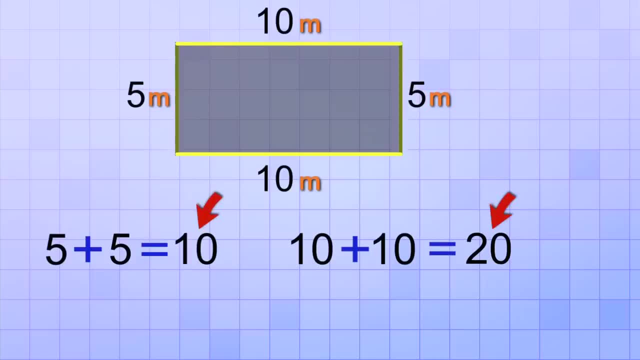 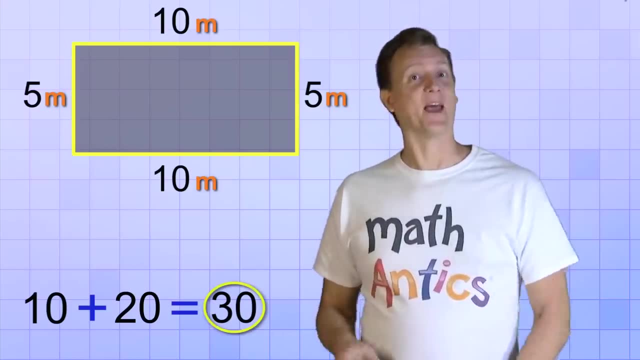 And now, if I add up those two answers, I'll get the total for all four sides. 10 plus 20 equals 30. So the perimeter of this rectangle is 30. Meters- Ha, You thought I was going to forget my units, didn't you? 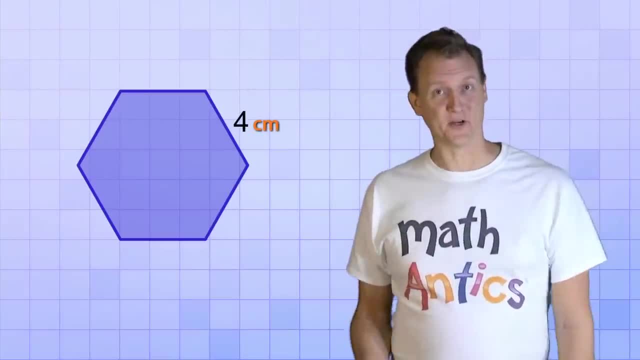 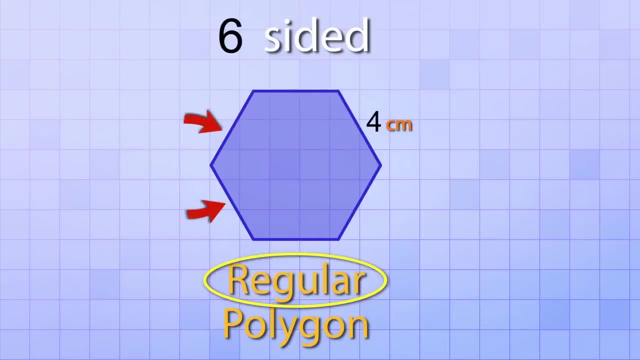 Not this time. Ah, here's another good example. This is a six-sided regular polygon. A regular polygon means that all its sides are exactly the same length, And that's good, because this diagram only shows the length of one side: 4 centimeters. 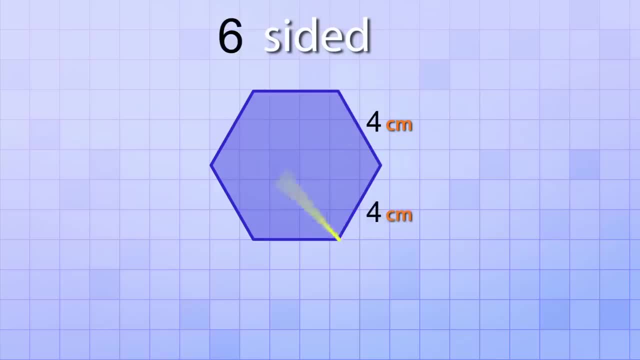 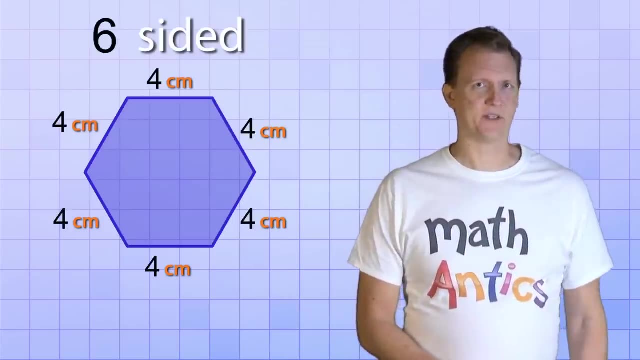 But since the polygon is regular, we know that all the other sides are also 4 centimeters long. Now we could just add up all the sides, like we did before, but since they're all the same, we can use multiplication as a shortcut. 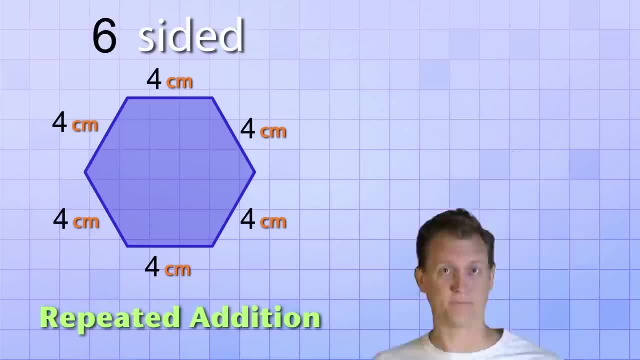 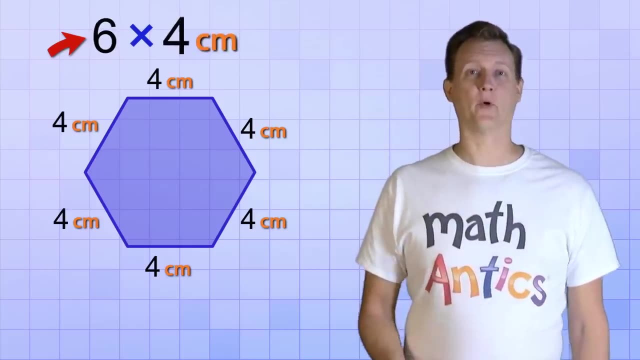 That's because multiplication is really just repeated addition. All we have to do is multiply the number of sides- 6, by the length of the sides- 4 centimeters. 6 times 4 equals 24.. So that means the total perimeter of the polygon is 4 centimeters. 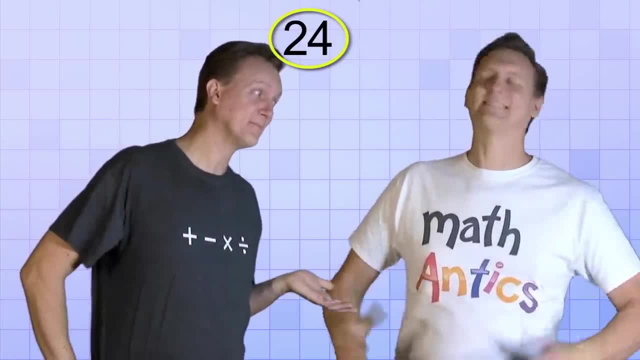 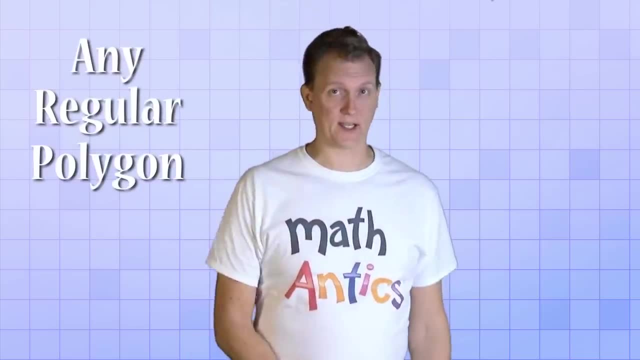 So the total perimeter must be 24.. 24, what Centimeters? That's better, Oops. And this formula works for any regular polygon, no matter how many sides there are. If the sides are all the same length, you can just multiply the number of sides by the side length. 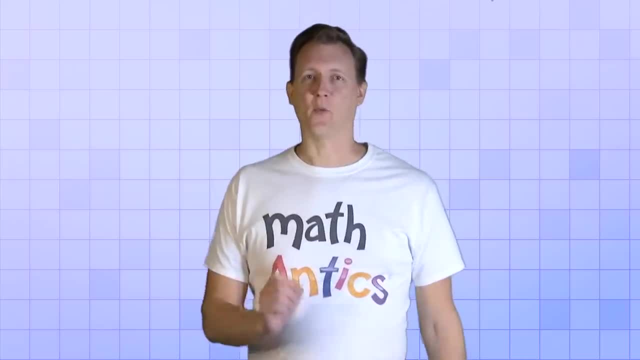 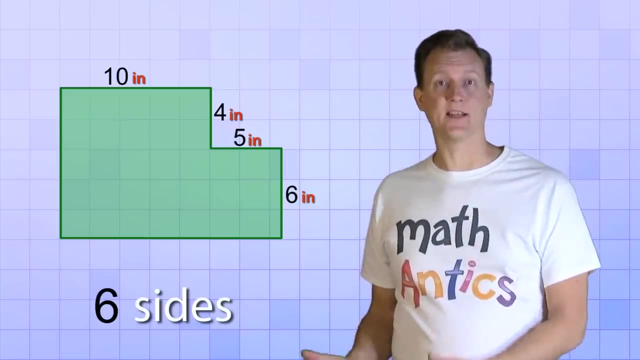 and you have the perimeter. Okay, let's try one more example. This polygon also has 6 sides, but it's not a regular polygon. The sides are different lengths, and this one's really tricky because they only show us the length of 4 of the sides. 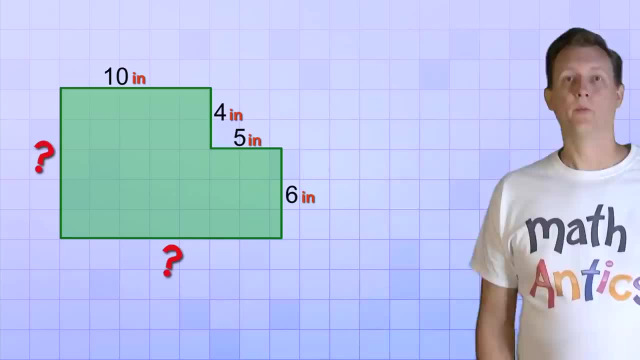 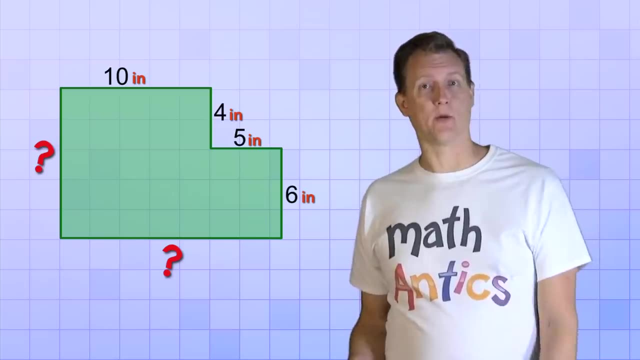 The other two are missing, So how can we figure them out? Problems like this come up all the time in math Problems where you aren't quite given all the information. When you have this kind of problem, the key is to use what you do know to figure out what you don't know. 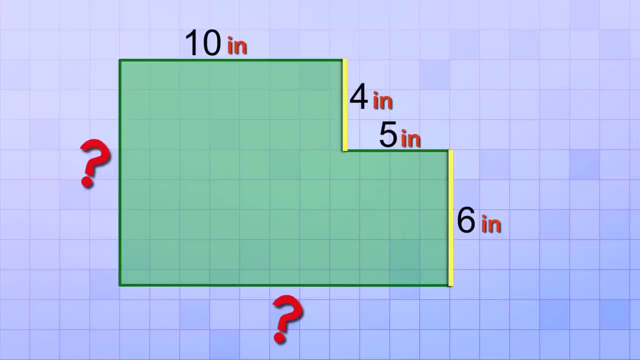 Here's what I mean. Look closely at the two vertical sides that we do know, the length of 4 inches and 6 inches. Now imagine that those two vertical sides could be moved straight across To the other side, The side that we don't know the length of. 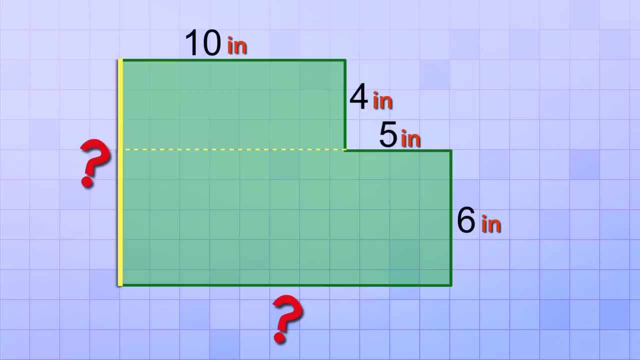 By doing that, you can see that the missing length would just be the combination of the two vertical lengths that we do know, 4 inches and 6 inches. And since 4 plus 6 equals 10, the missing vertical side must be 10 inches long. 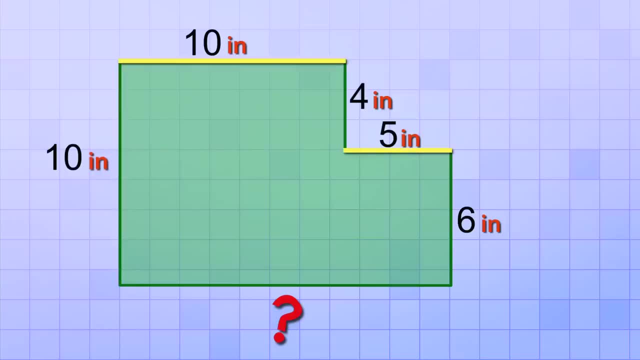 Notice that we can do the same thing for the horizontal sides that we do know. If we imagine those moving down to the side that we don't know, we see that its length must be equal to the combination of those two lengths. 10 inches plus 5 inches equals 15 inches. 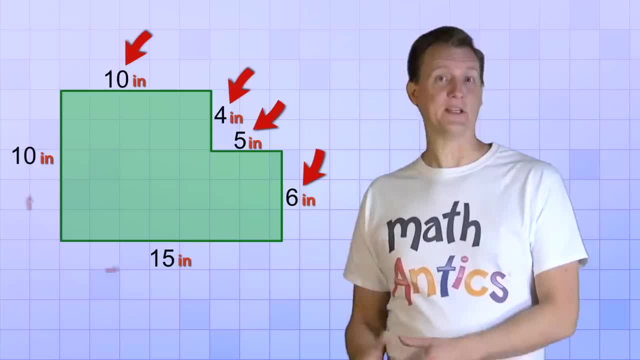 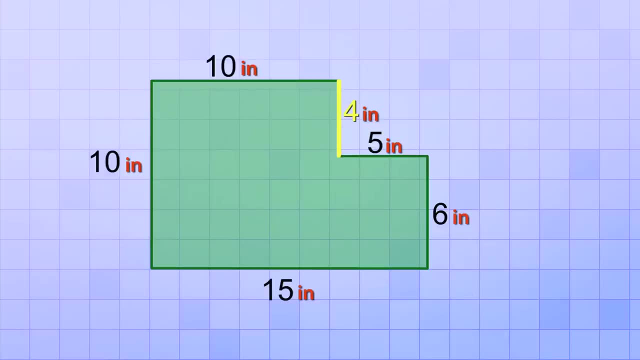 There we've used the lengths that we did know to figure out the lengths that we didn't know, And now that we know the lengths of all the sides, we can just add them all up to get the perimeter. 4 plus 5 plus 6 equals 15.. 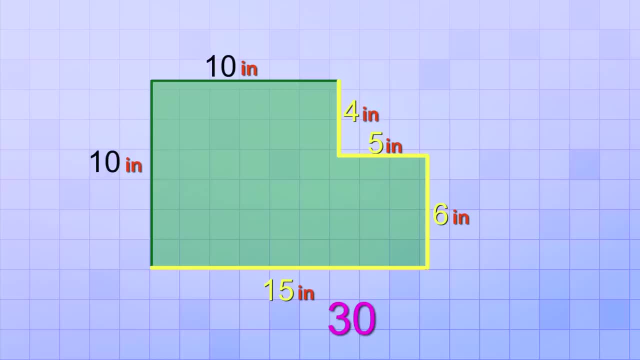 And then 15 plus 15 equals 30.. 30 plus 10 equals 40. And, last of all, 40 plus 10 equals 50. So… the sum of all the sides is 50 inches, And that's the perimeter of this shape. 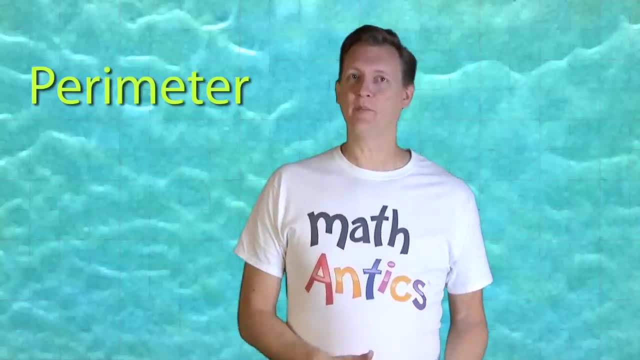 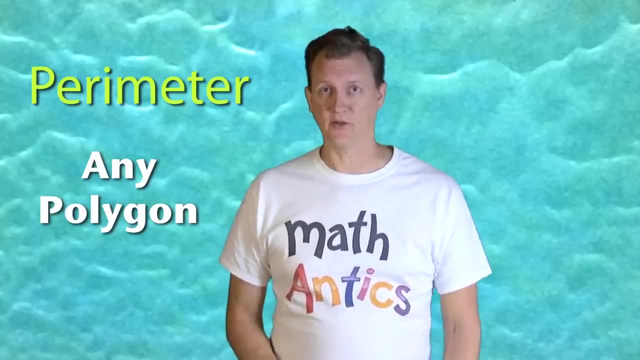 And that's the end of this lesson. We've learned that perimeter is the distance or length around a geometric shape, And we've learned how to calculate it. for any polygon, You just add up the lengths of all the sides and the total length is the perimeter. 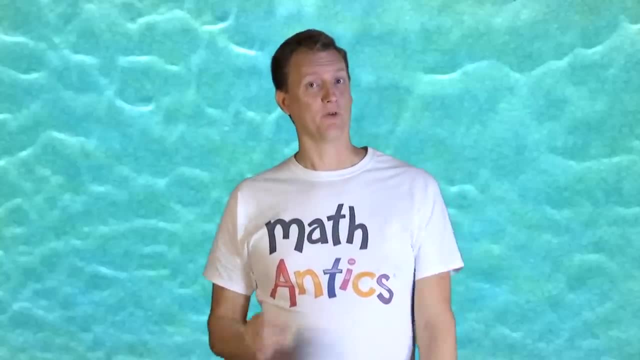 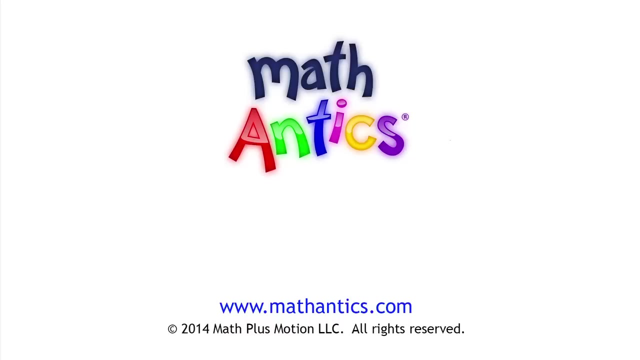 Oh, and don't forget your units. Also, don't forget that to get good at math takes practice. Thanks for watching Math Antics and I'll see you next time. Learn more at wwwmathanticscom. 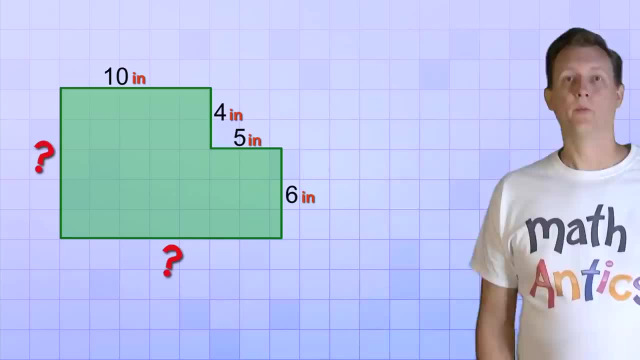 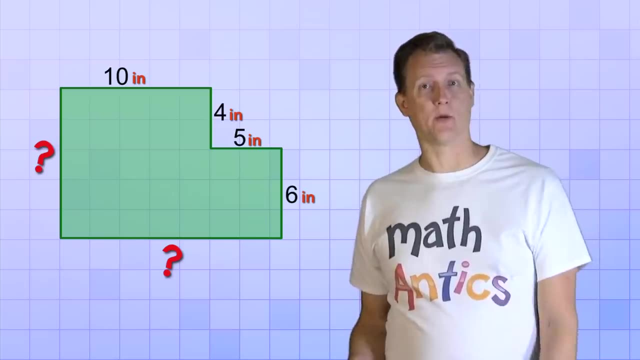 The other two are missing, So how can we figure them out? Problems like this come up all the time in math Problems where you aren't quite given all the information. When you have this kind of problem, the key is to use what you do know to figure out what you don't know. 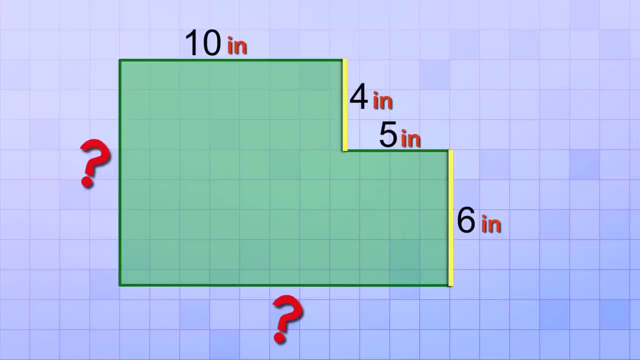 Here's what I mean. Look closely at the two vertical sides that we do know, the length of 4 inches and 6 inches. Now imagine that those two vertical sides could be moved straight across To the other side, The side that we don't know the length of. 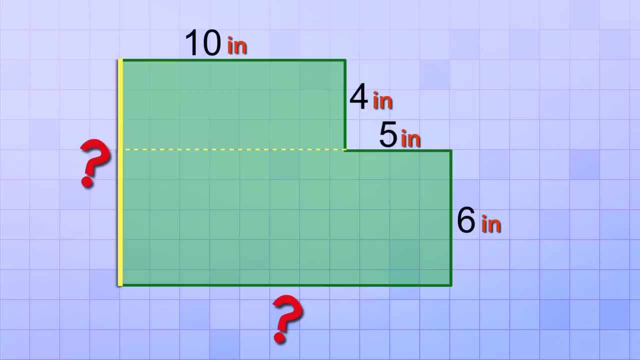 By doing that, you can see that the missing length would just be the combination of the two vertical lengths that we do know, 4 inches and 6 inches. And since 4 plus 6 equals 10, the missing vertical side must be 10 inches long. 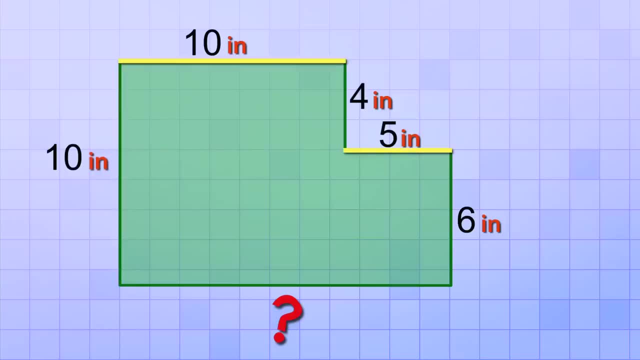 Notice that we can do the same thing for the horizontal sides that we do know. If we imagine those moving down to the side that we don't know, we see that its length must be equal to the combination of those two lengths. 10 inches plus 5 inches equals 15 inches. 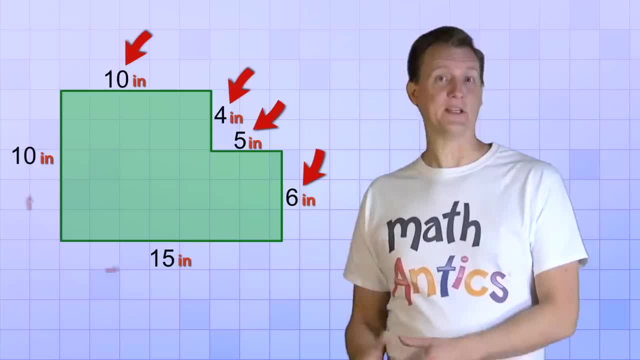 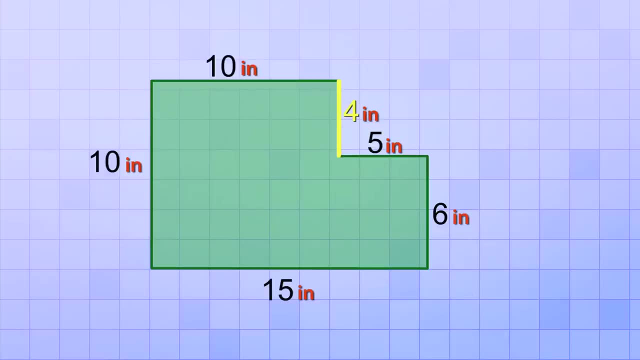 There we've used the lengths that we did know to figure out the lengths that we didn't know, And now that we know the lengths of all the sides, we can just add them all up to get the perimeter. 4 plus 5 plus 6 equals 15.. 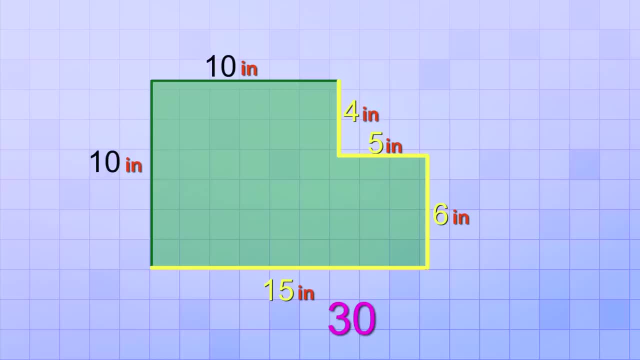 And then 15 plus 15 equals 30.. 30 plus 10 equals 40. And, last of all, 40 plus 10 equals 50. So… the sum of all the sides is 50 inches, And that's the perimeter of this shape. 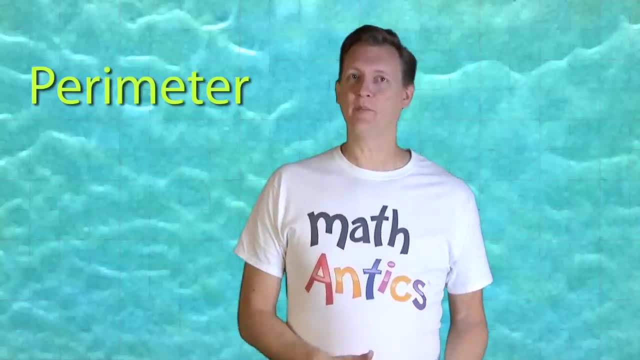 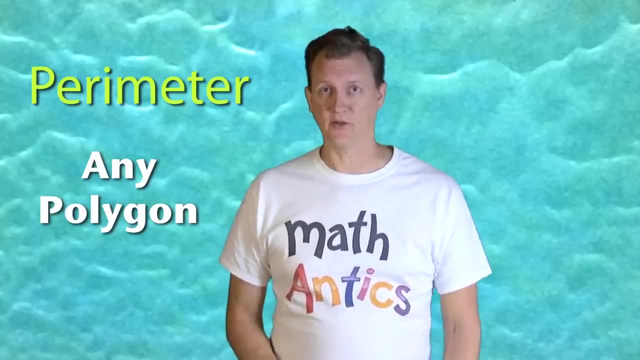 And that's the end of this lesson. We've learned that perimeter is the distance or length around a geometric shape, And we've learned how to calculate it. for any polygon, You just add up the lengths of all the sides and the total length is the perimeter. 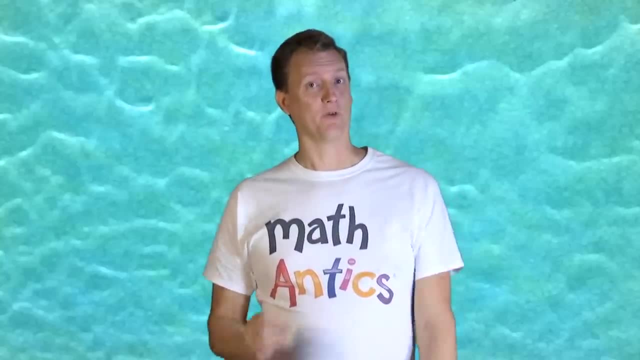 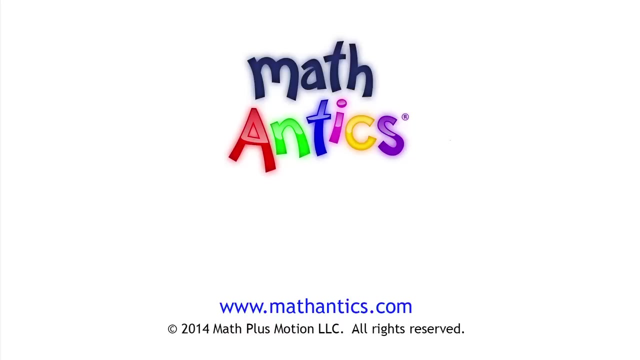 Oh, and don't forget your units. Also, don't forget that to get good at math takes practice. Thanks for watching Math Antics and I'll see you next time. Learn more at wwwmathanticscom.